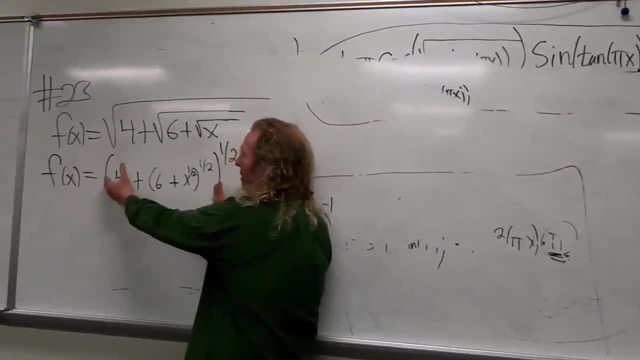 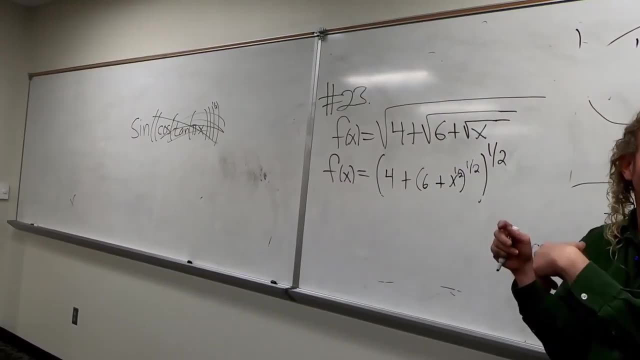 So notice how I work from the outside. in I wrote the one half down first, Four, the plus: this is this and this is this. So that's the hardest part, I think, is the rewriting. in my opinion, At least in my- I have a harder time with that. 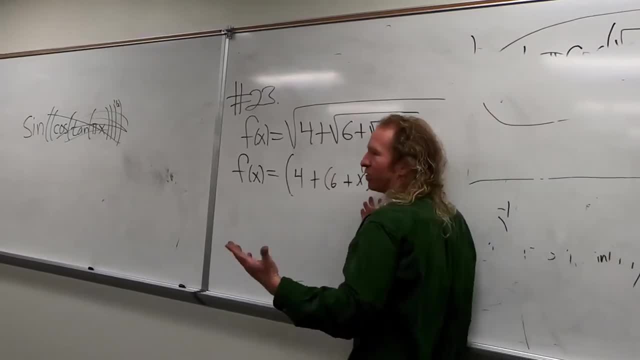 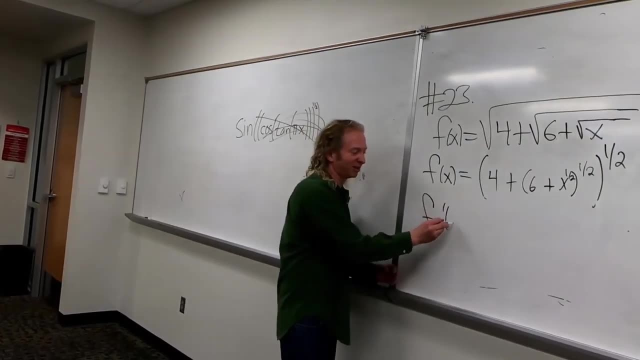 I have an easier time with a derivative and a harder time with this step for some reason, Then maybe that's not common, I don't know. Okay, so now we're going to take a derivative, So F prime of X. So you put the one half in the front Right, So one half. 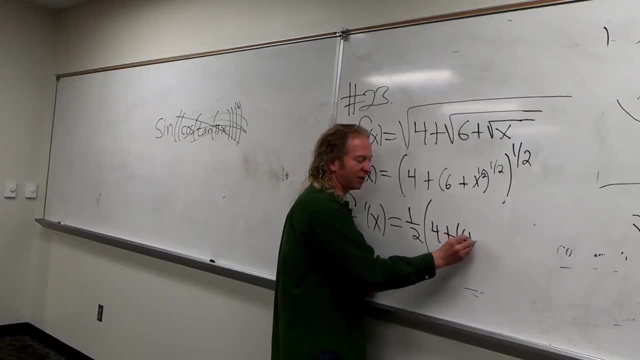 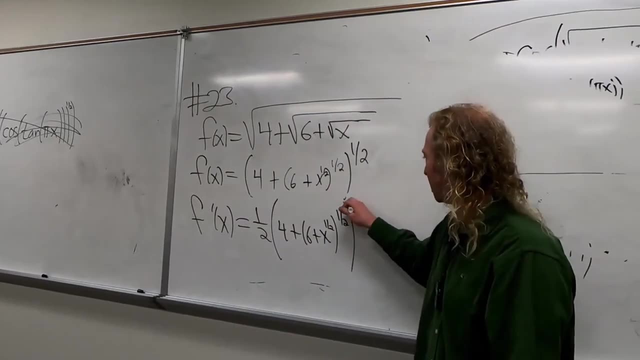 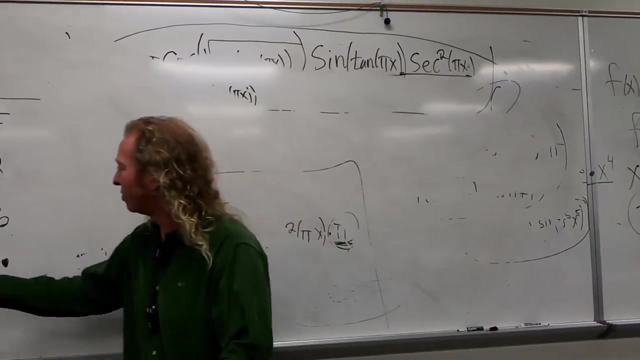 Parentheses four plus parentheses six plus X, to the one half, to the one half, Negative one half times the derivative of the inside Right. So this is zero. So in this one, So this is the chain rule right. So one half. 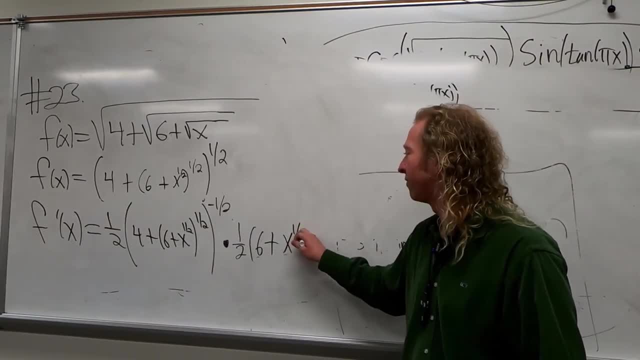 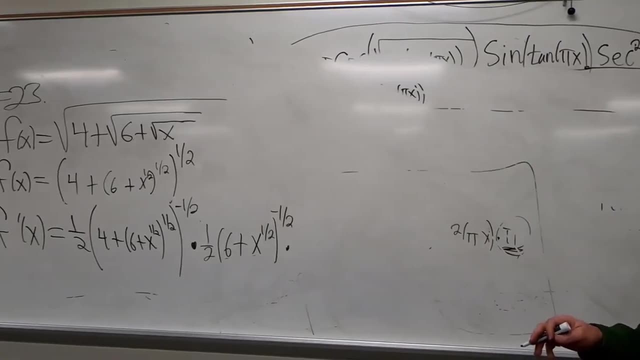 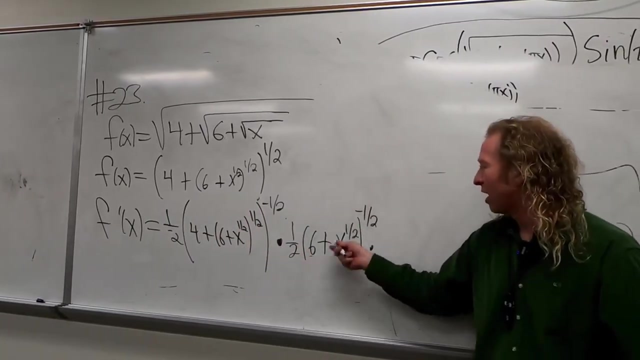 Six plus X to the one half, to the negative one half times. So let's see: So one half, Leave the inside untouched, Negative one half, Take this derivative And then we're taking this derivative. You do this Subtract one. 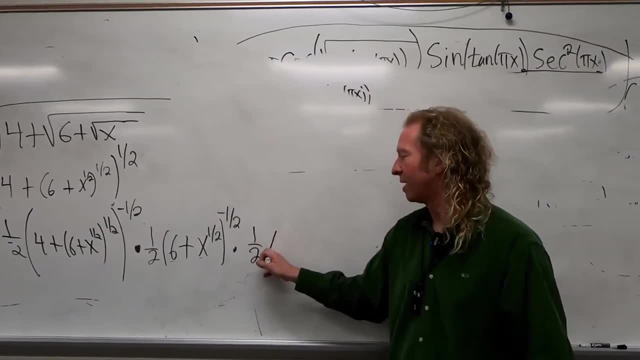 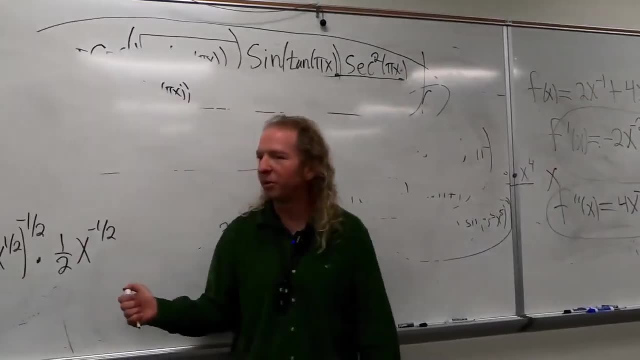 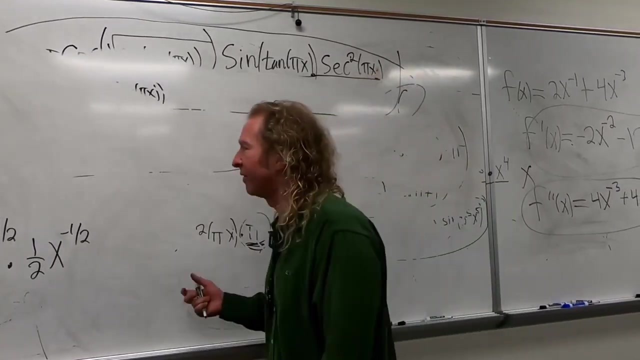 Now it's the derivative of this right, So one half, X to the negative, one half. So it's a little bit. Yeah, That's fine. Yeah, it's fine. Now we're going to simplify it. It shouldn't be too bad, I hope. 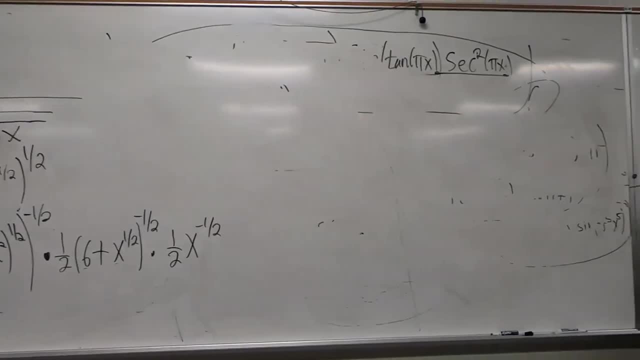 But let me go over it again. We still have like three minutes. That's good. We still have two minutes, A minute and 55 seconds. Okay. so we have this to the one half. I put the one half in the front, So we're here. 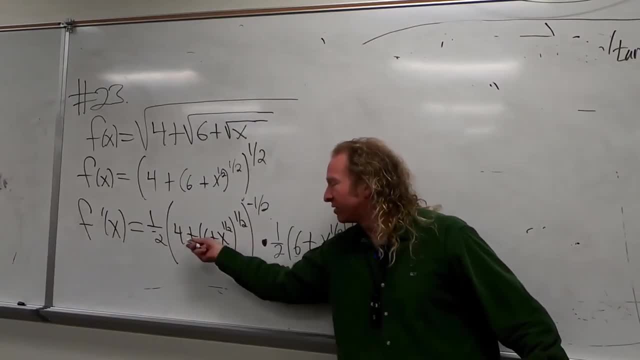 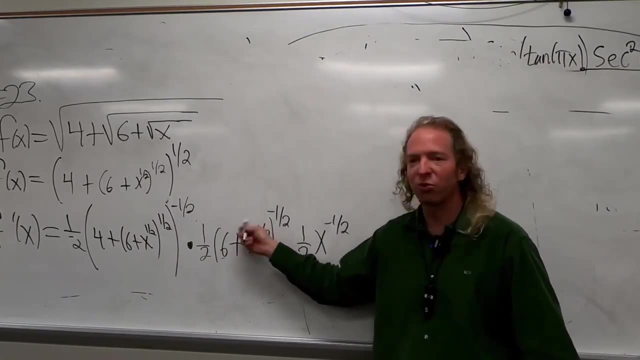 Subtract one: Okay, And then take the derivative. Take the derivative of this. This is zero. So this derivative here, it's one half. Leave this untouched. Subtract one: You get here. Take this derivative here, This is zero. 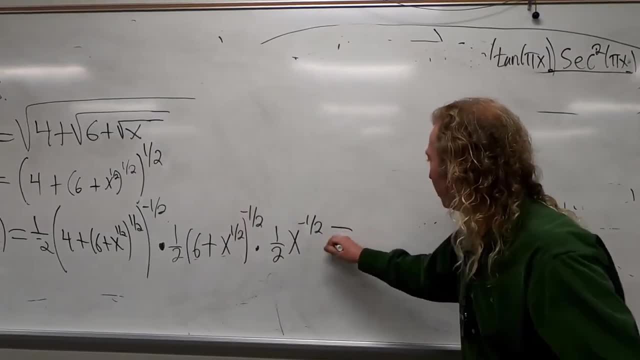 This derivative. here is one half X to the negative one half. So we're good, Let's clean it up. I'll do it here. So I think it's going to be a fraction. Wow, Almost everything is going to go downstairs, right. 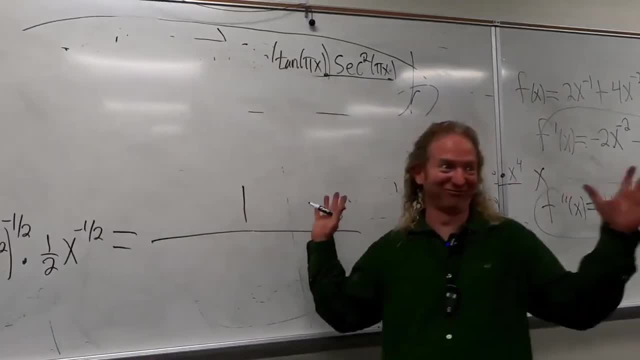 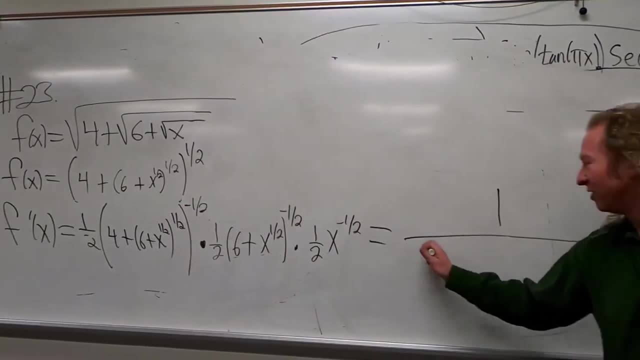 Wow, It's ridiculous. Okay, So we have one. It's ridiculous, It's all going down. Oh look, Two times two times two is eight. We can have an eight here, And then this is a giant square root on the bottom.